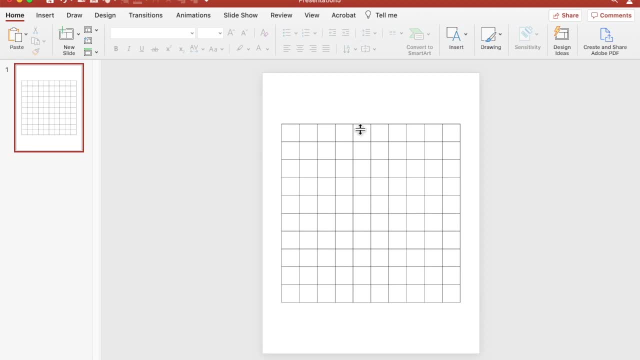 all four quadrants on your grid. all you would have to do is select your table, go to table design and then, for borders, you're gonna hit on the pen color and then pick the color you want. i'm just gonna choose black and then i'm gonna go down the line and then it highlights that line and then 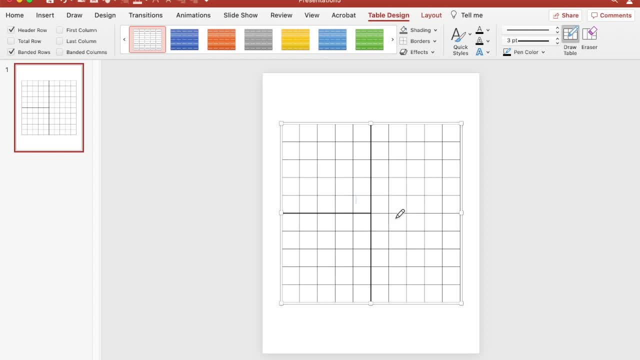 i'm going to click here for the line to go across. let's undo that one hit the pen again and then you can make it thicker or thinner, and then you can add a line here like: so we're gonna change it. i'm going to change it to a. 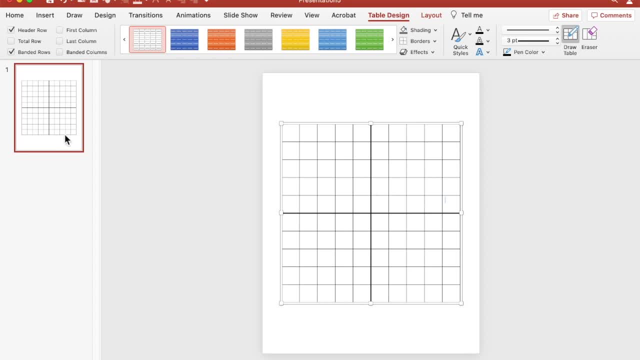 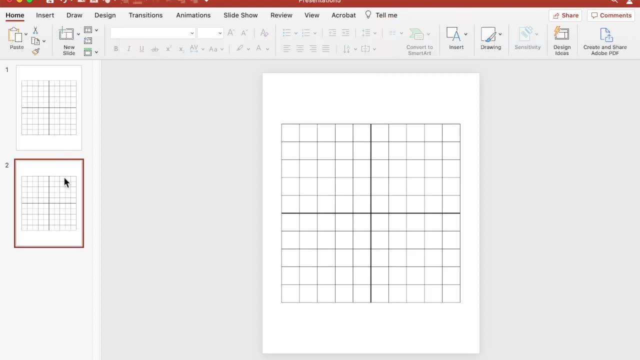 little bit thicker, and then i'm gonna come over here. where it changes, it adjusts the weight of the line, so that's, if you want it all for quadrant. so i'm going to duplicate this page. i'm going to come over here and duplicate the page and leave that for quadrant. so now, 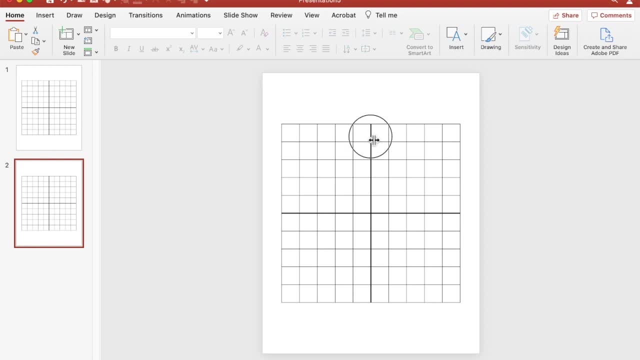 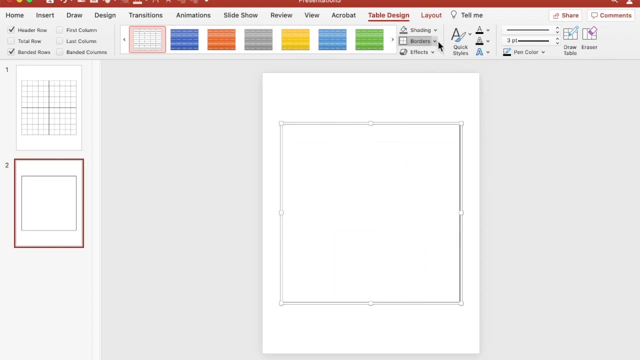 because i work with elementary students. we only work in quadrant one, when we're focusing on table design, and then for borders, I'm going to put no border, all border. I want to be one point, then we're going to put that in there. so now I want the outside. 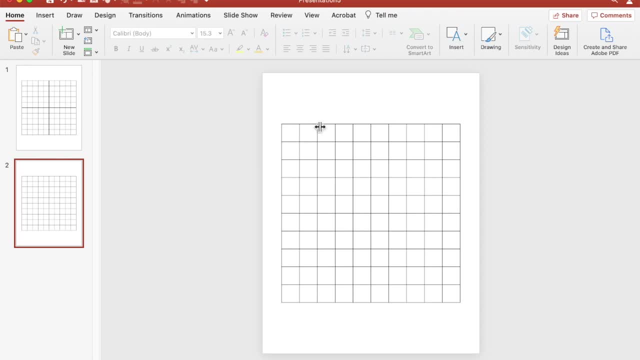 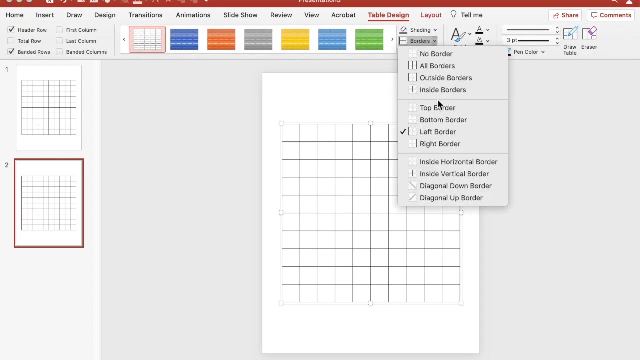 of the grid, the left border to be darker or to be highlighted. so I'm going to hit three point and then I'm going to hit left border so you can see it's darker, and then I'm going to do the same thing for the bottom border. so I wanted those. 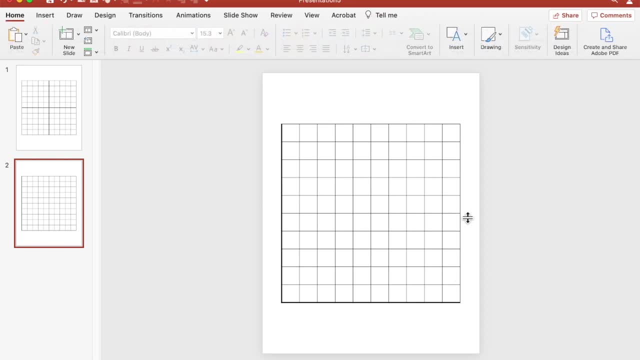 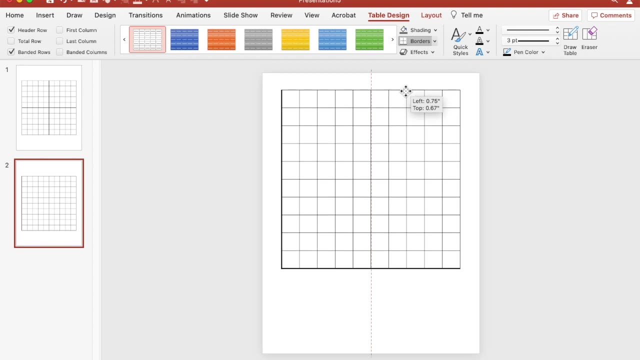 two parts of the grid to be highlighted. the next thing I'm going to do is add in my numbers. so at this point I do want to move the grid up and I'm going to add in little text boxes where I'm going to add in my. 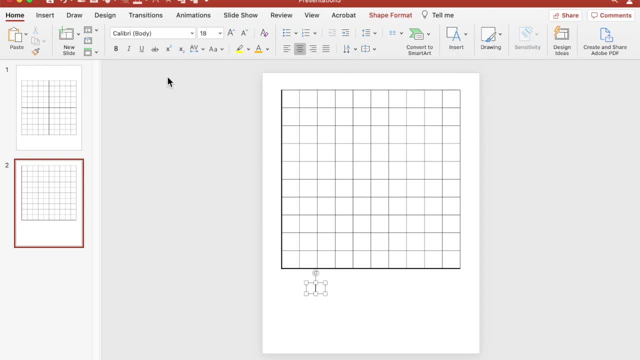 numbers, and then I'm going to hit left border. so I'm going to hit left border number, so I'm going to Center it, put it in the middle of the box and then choose the font that I want. so I'm going to put zero here and then adjust the text box. 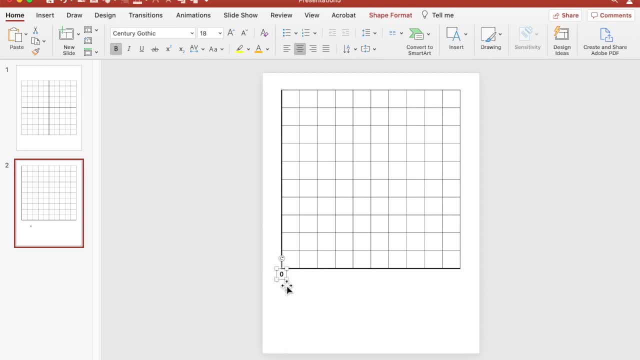 and I'm going to put the zero here for now. I'm not going to leave it there because I need a zero on the x-axis and the y-axis and I'm just gonna have one in the corner, but for now I want that zero there to help me align my numbers. 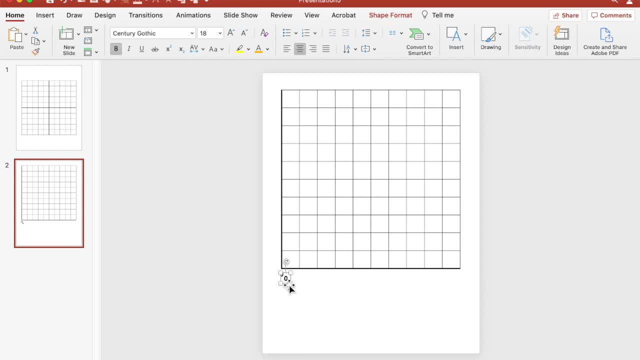 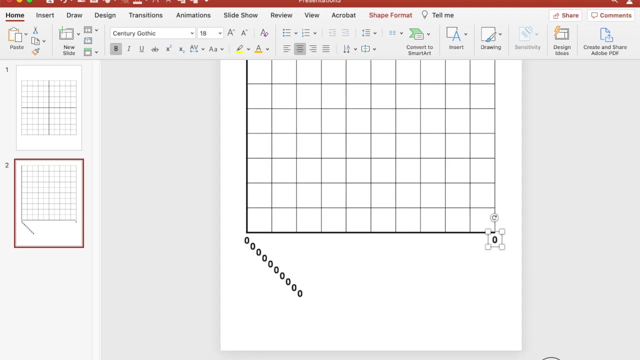 on the bottom. so I'm going to duplicate the zero ten times. so I am going to bring this over here. I want it to be lined up and if it's too small for you to see this, zoom in on your page, all right. so these are these. two zeros are aligned. so now. 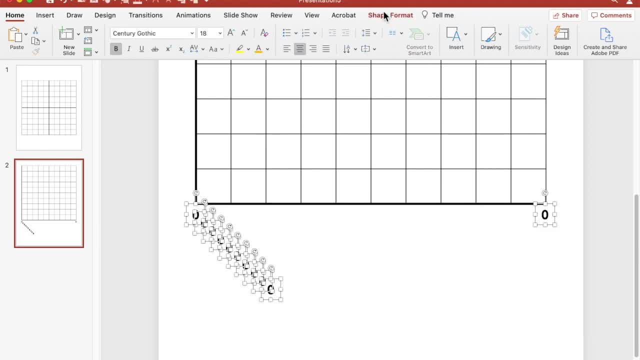 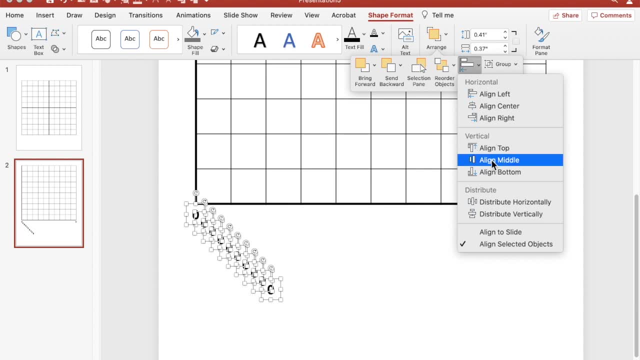 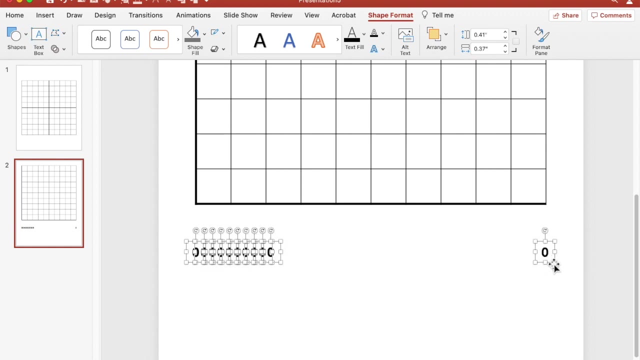 what I'm going to do is select all of the text boxes, go to shape format, arrange, hit align and then hit align middle so that they all line up together, and then let's move that up. and then I'm going to go back to a range, hit align and then 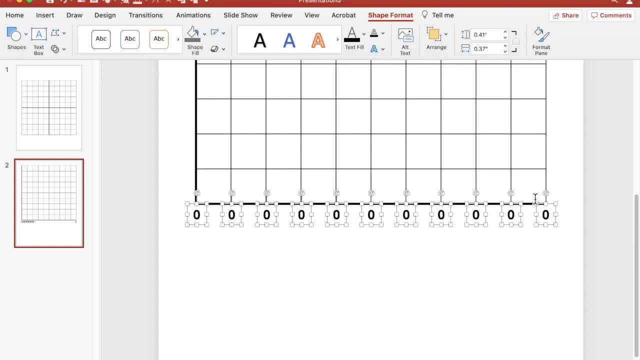 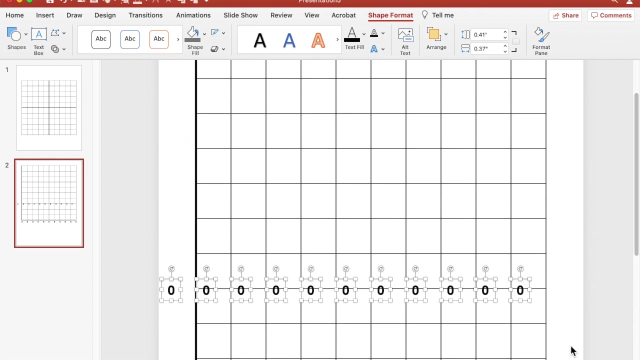 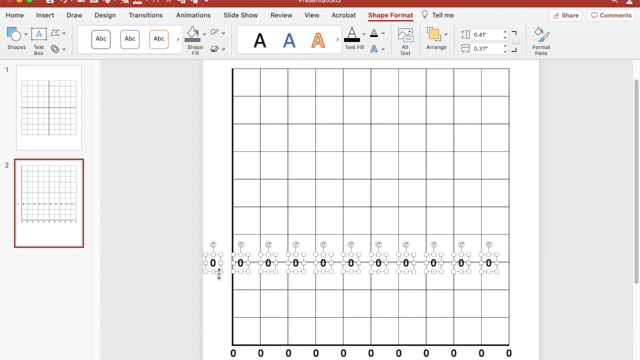 hit, click on distribute horizontally. so hopefully they are all pretty much lined up with their line. and then I'm going to do the same thing: select those, duplicate it and move those up. let's go up the page and zoom out a little, and now I'm going to unselect and 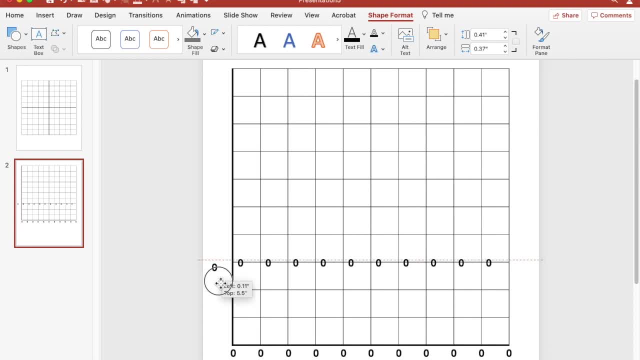 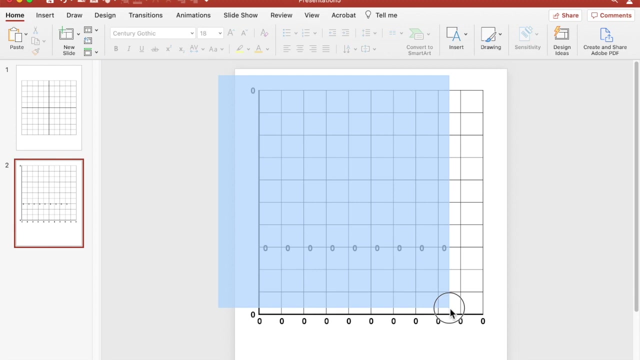 then select one, put that zero there And I'm going to put the zero up here and make sure it's lined up with the zero at the bottom And then I'm going to select. let's zoom out a little bit more. I'm going to select all of them and try to get that zero at the bottom. 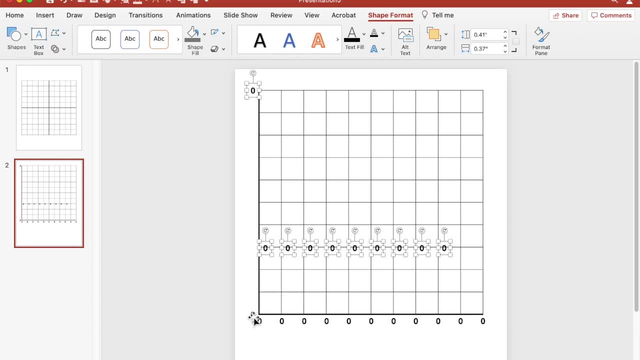 If it's not selected, just hold down your command key or control, if you have a PC, and then select that zero. So I'm going to go back to arrange align. let's do align left. there we go. Now they're all aligned vertically. now I want to distribute vertically evenly. 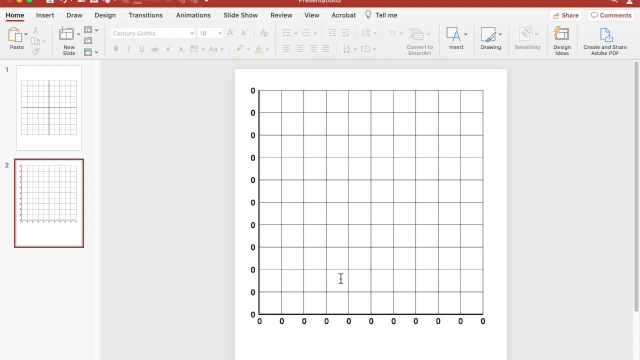 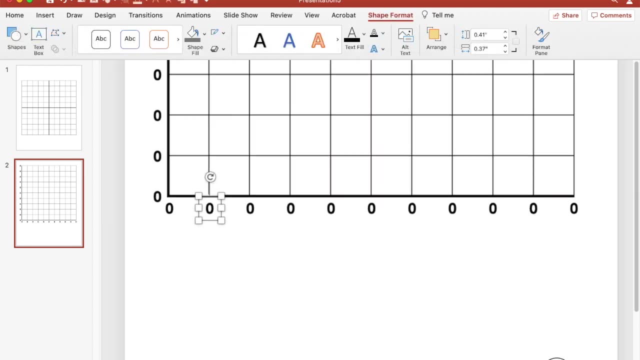 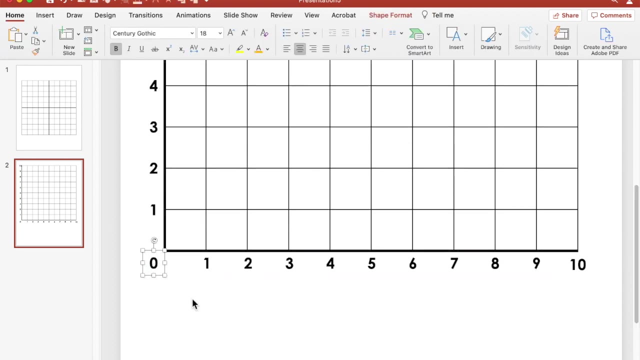 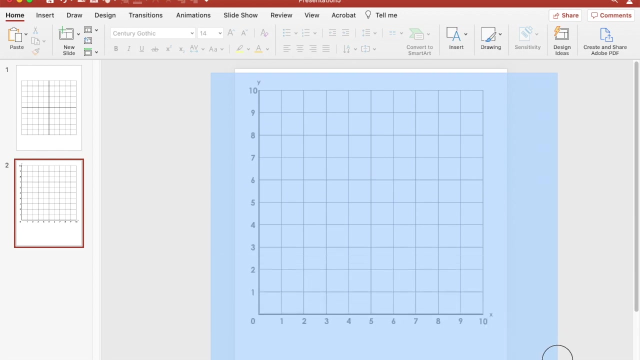 So now those are all lined up with those lines. okay, So now what we can do is adjust our numbers. So this one- I'm going to zoom back in- it's going to be one. So now I'm going to group my numbers together just to make sure nothing gets moved around. 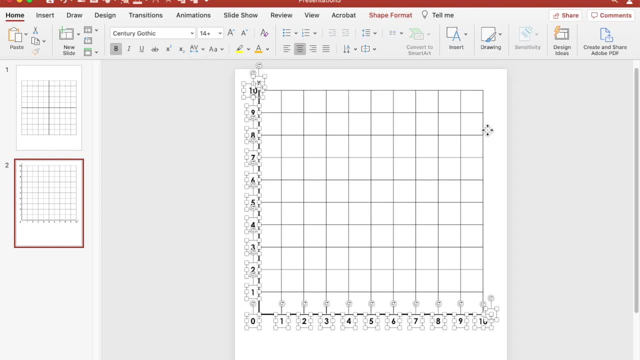 So I selected them all. I can't group it with a table because for some reason, tables you can't group them. So I unselected the table, but I'm going to right click with everything else and group them together. So now my numbers are together. 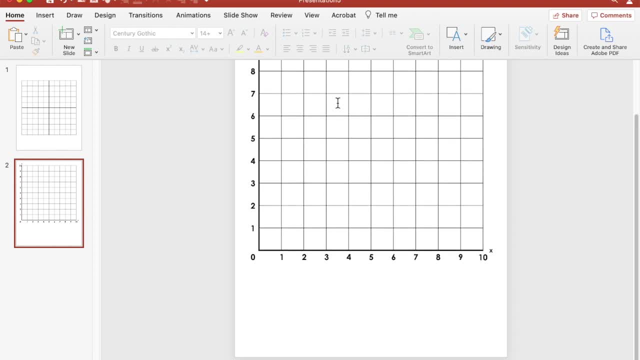 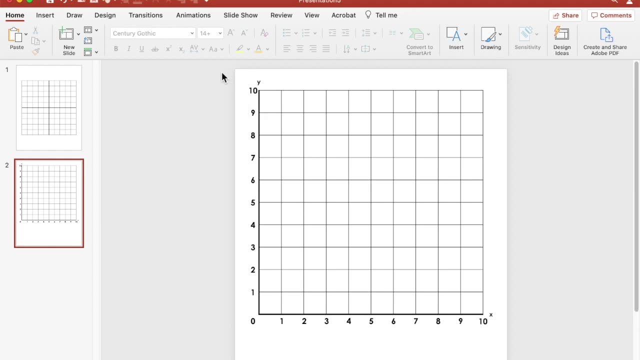 So now for this first page. I don't want anything to be on the grid. I want it to be blank, because I want my students to plot the points on the grid. So I'm going to save this image as a picture, just the way it is. 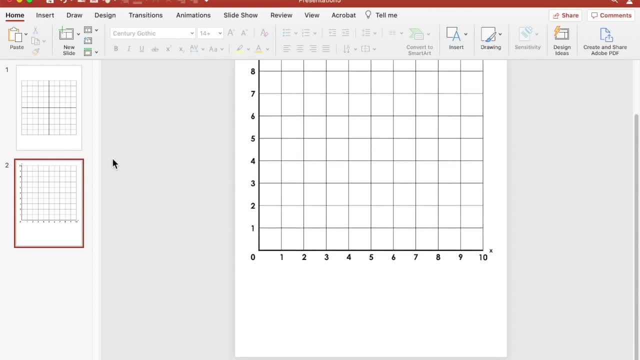 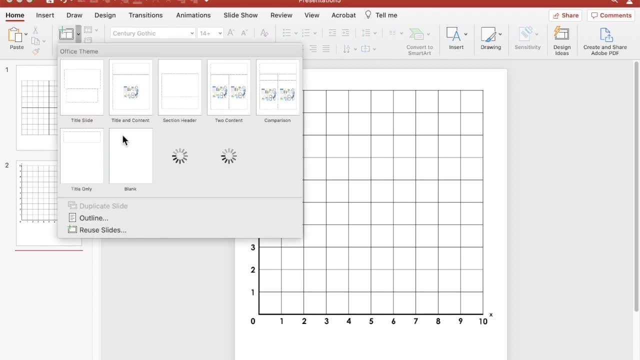 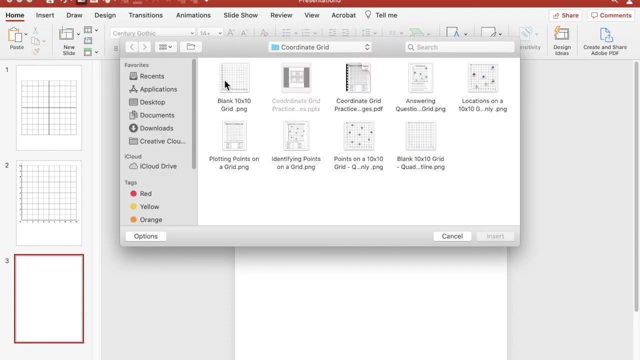 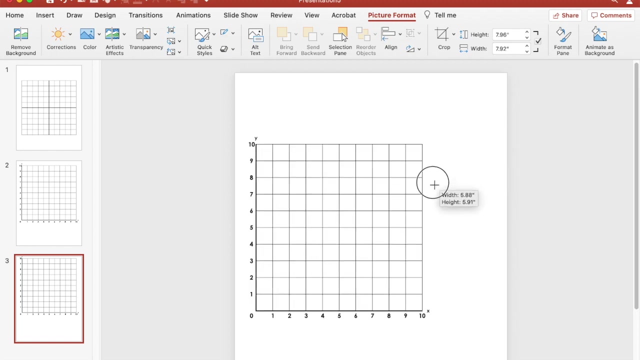 Put that there. So now I can add on. So I'm going to add on to a page, So I'm going to start a new page And I am going to insert my image that I just created blank 10 by 10 grid, and now I can shrink it and move it around however I want, without the features of the image getting distorted or messed up. 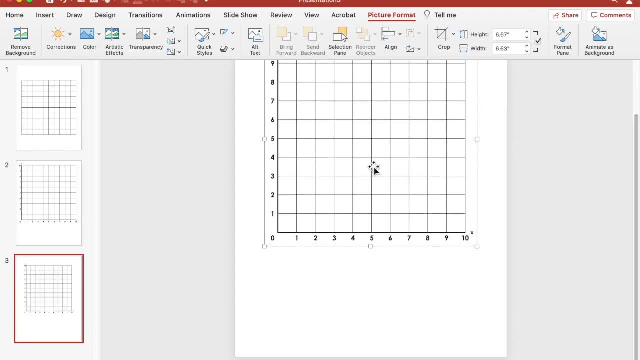 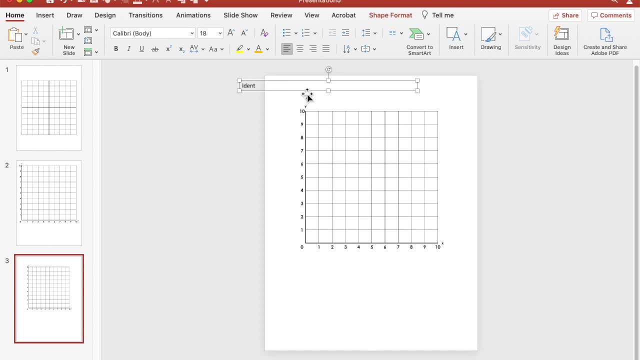 All right, so there is our grid. Now we can add questions for our grid. So for this first page, I want them to plot points on a coordinate grid. So we have our basic heading name and our title and then we have our grid plotting on a coordinate grid. 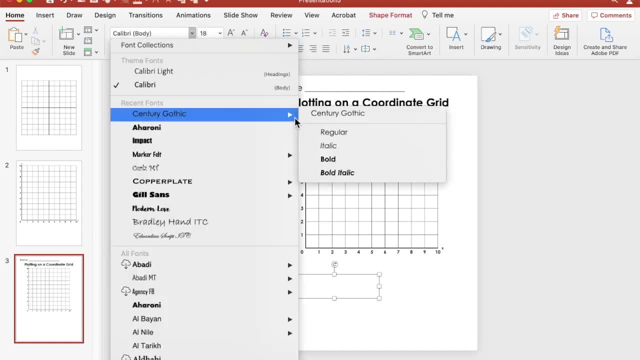 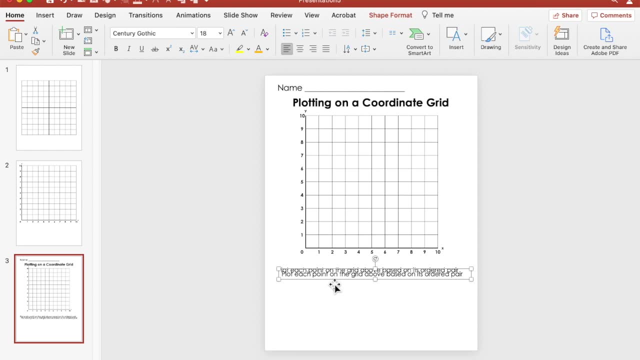 Now we're going to add in a text box. Those are the instructions. Now let's put in the actual points that they're going to use, And I do want these to be bold, So I'm going to add in a text box. 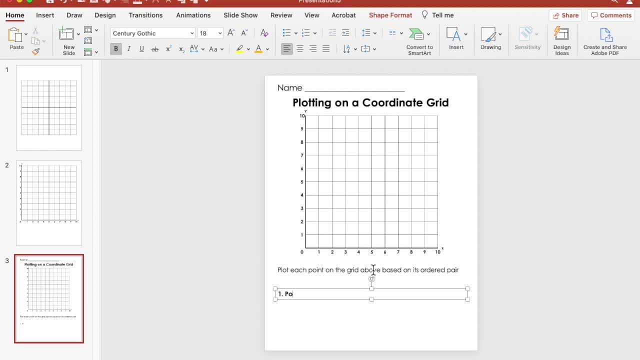 So I'm going to add in a text box. So let's start with number one. So if I have point A, where is point A going to go? So one thing you can do: you can make these up, but you might get mixed up with where you're putting something. 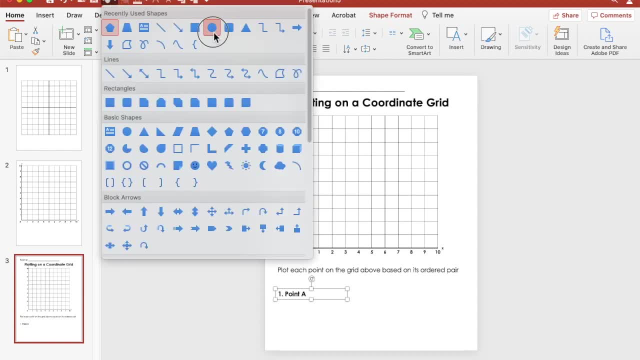 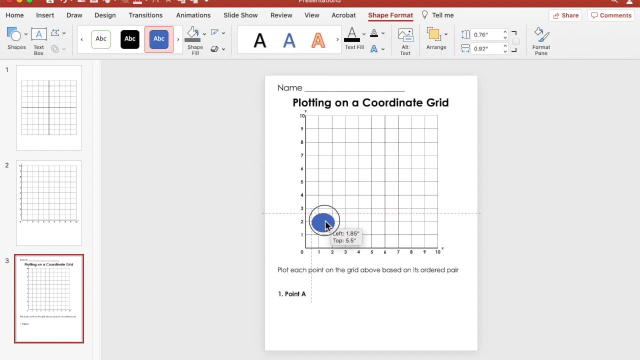 So I'm going to draw a shape, I'm going to draw a circle. Let's put that circle. let's say 4, 6. maybe That's a little bit too big. Okay, so that's where my point A is going to go. 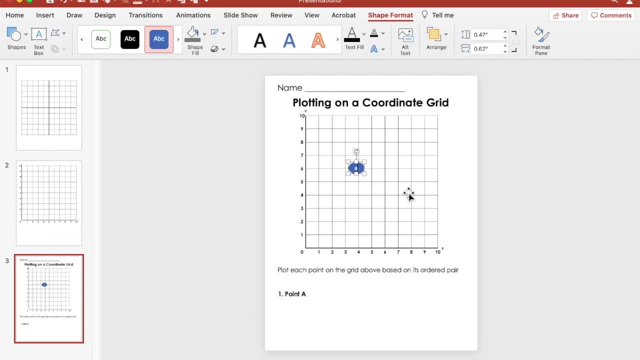 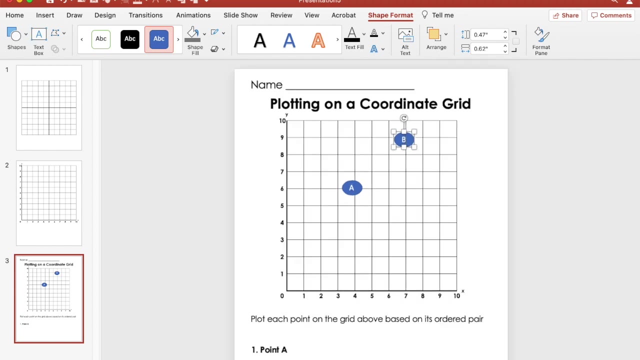 And actually you can type in there. So that's point A. Let's see where am I going to put point B. Let's put it here And change that to B. Let me zoom in a little bit, So I just want to plot these points so that I know where I want to put my points. 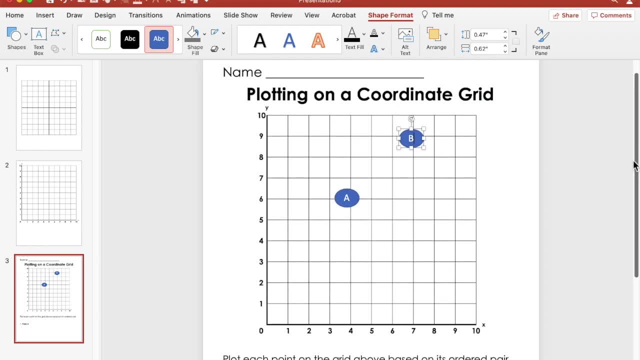 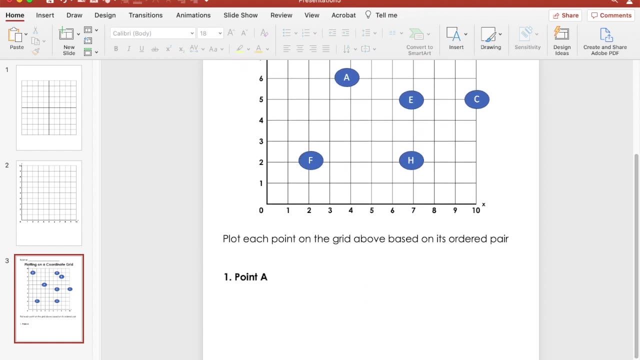 And then I'm going to add coordinates down below for the students to plot later on. So I'm going to duplicate that For point C. let's put one here. Alright, so we have our points, and now we just need to put in our clues at the bottom. 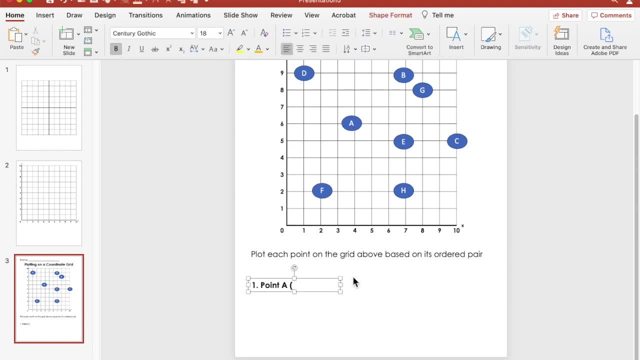 Or our points, our ordered pairs. Take the bold off. So point A, we said, is F, 4, 6. Let's put a space 4, 6. And then we're going to duplicate these. So there's 8 points. 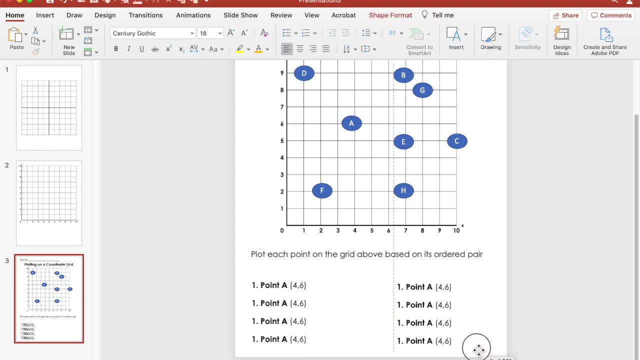 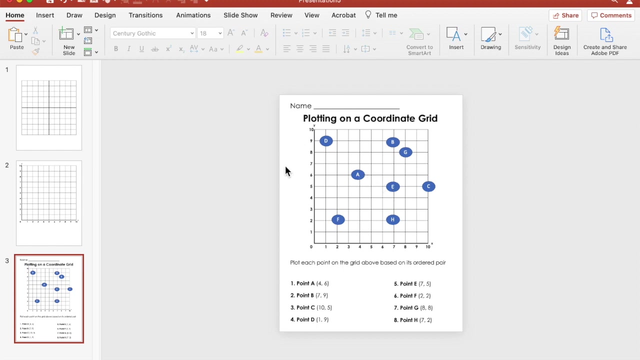 So I have that, And then I can duplicate that set and bring that over here And just line it up. Alright, so number 2. Which is B, And B is at 7, 9.. So now we have our clues or our questions to go on here. 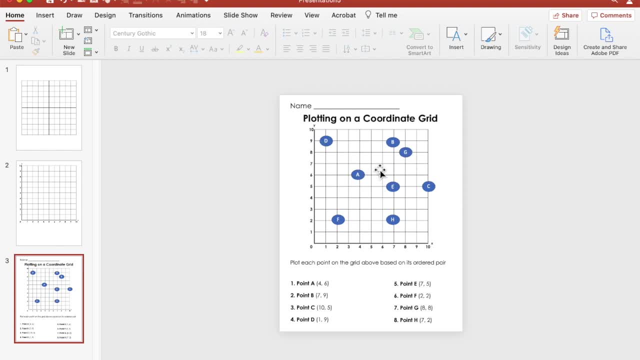 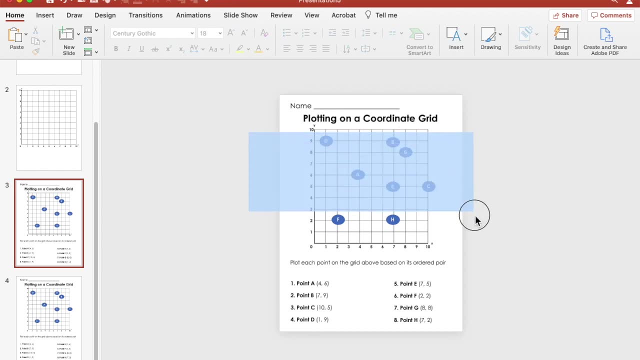 So I want to keep these circles for the next page that we're working on, So I'm going to duplicate that and come back here. So now, what I'm going to do is I'm going to duplicate that, So what I'm going to do is delete those circles, because I want the students to plot those points on the grid. 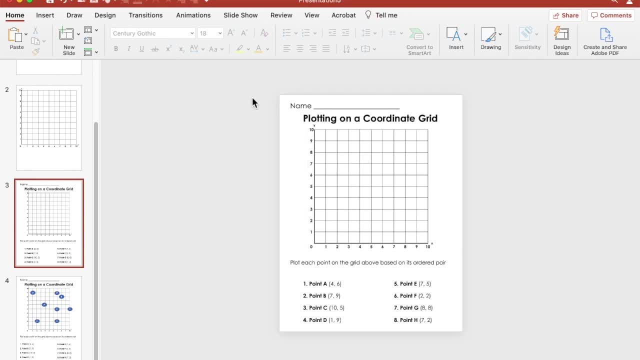 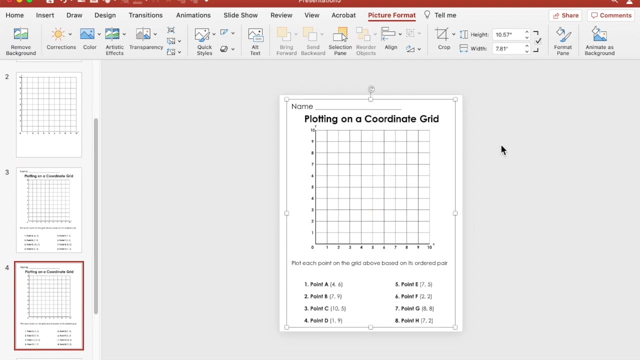 We already saved the grid as an image. What I want to do now- this is optional for you- is to save the entire page as an image. So go to save as Save. So we have our image. We have the one we were editing. 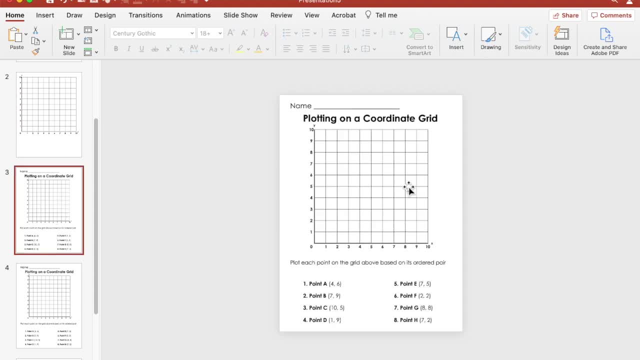 And we have our original grid that we made. So with the one that you're editing, you want to keep it. You don't want to get rid of it, even though you made the PNG image, Because if you want to adjust something, you always have that copy. 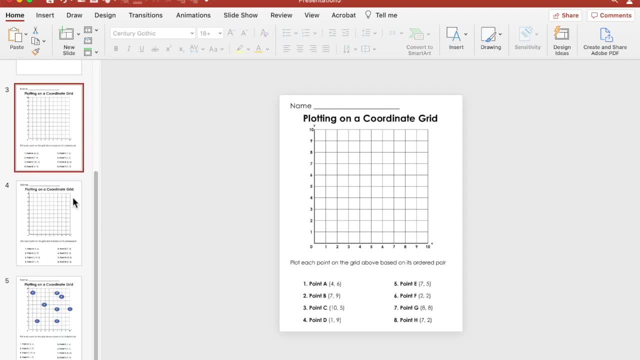 As a PNG, you can't make changes to that PNG, So you want to leave your blank copy. Alright, so let's move on to our next page. This time we're going to have the images or our points on the grid. 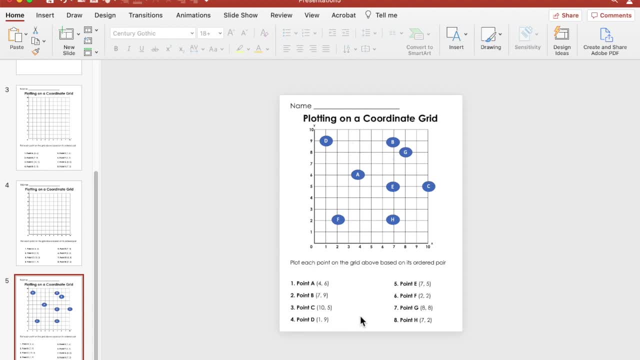 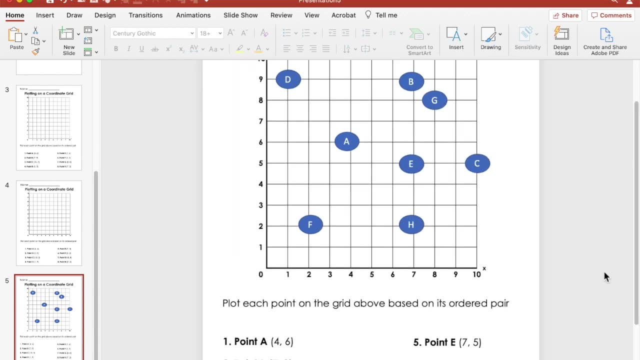 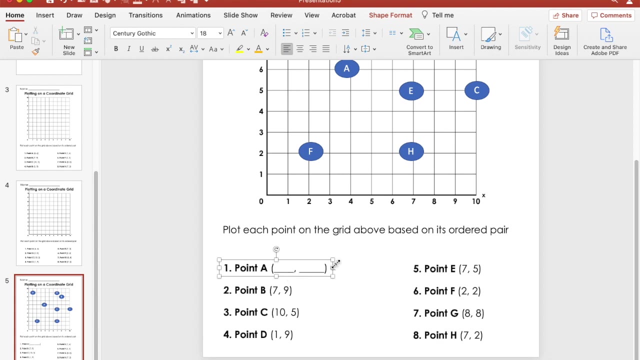 And then we're going to have the students figure out what these points are or what their coordinates are going to be or what the order pair is. So I'm actually going to delete what's inside and leave a blank space so they know that they need to write on it. 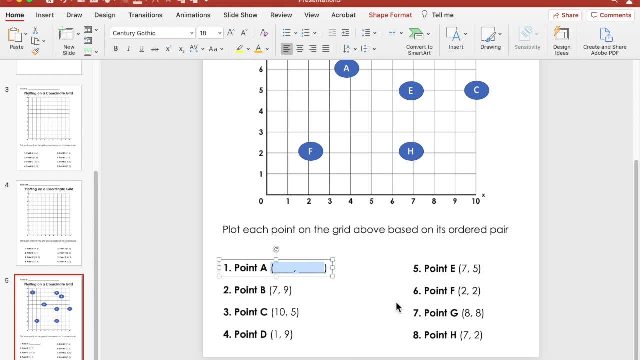 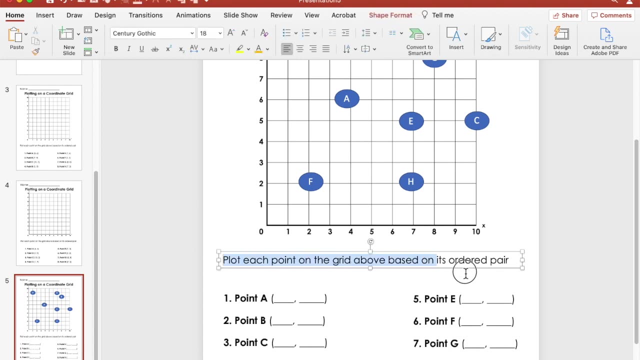 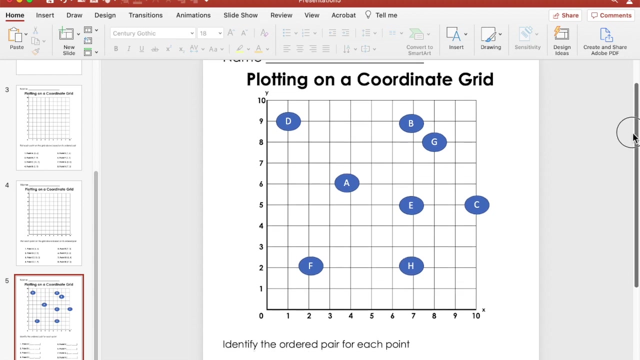 Let's just copy that inside section Copy Paste. So we have our grid Points and our blank coordinate pairs or ordered pairs at the bottom. So we need to change our instructions. So now you can leave them. But if students are working on the last worksheet, you don't want it to be exactly the same. 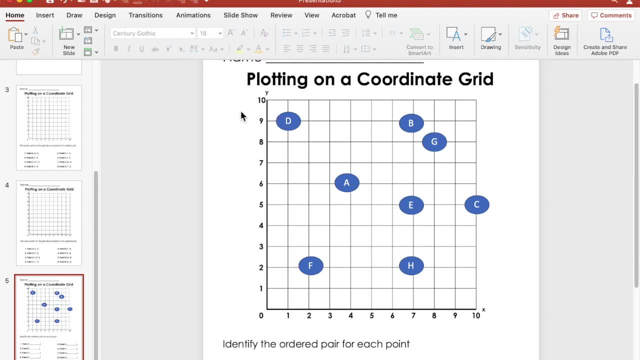 So I'm just going to move these around, And I actually want to adjust the dots to look like circles, So I'm going to do these over. So let's find our circle again. If you hold the shift button down, it makes that perfect circle. 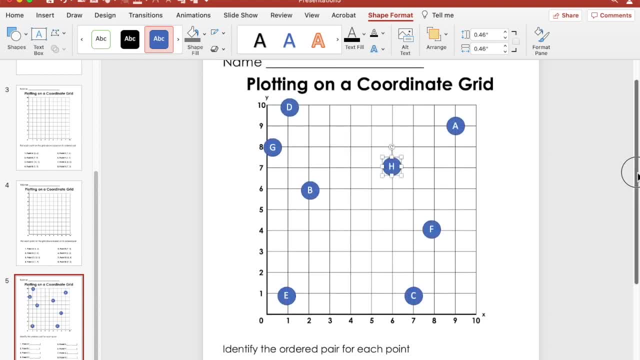 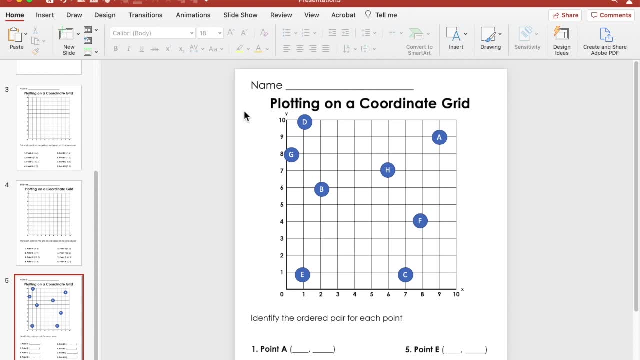 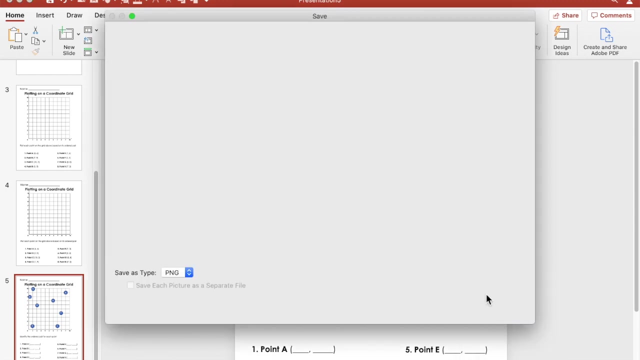 So we have our coordinate grid now with the images on there. So again, I want to save the grid by itself as an image. Let's make sure we have that table in there, Make sure you have all your letters selected, And we're going to save it as a picture and save. 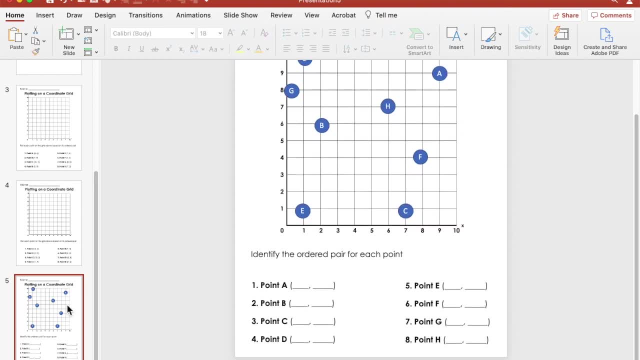 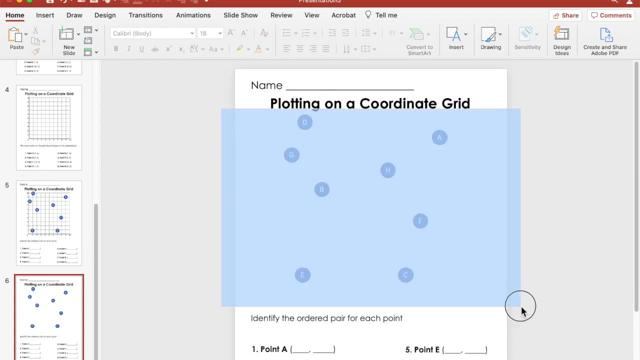 So we have that image saved. So now I'm going to duplicate this page And I'm going to get rid of the edited one And I'm going to insert the image- so everything is together- And again adjust the size to meet the needs there. 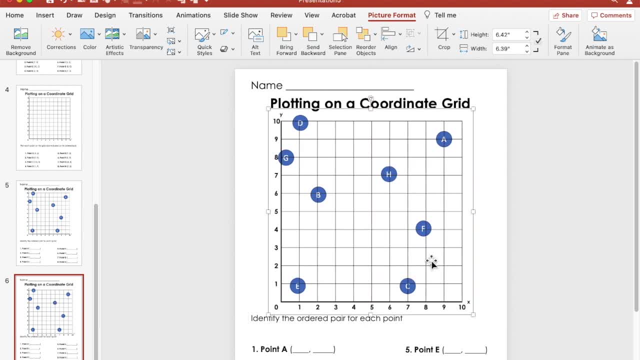 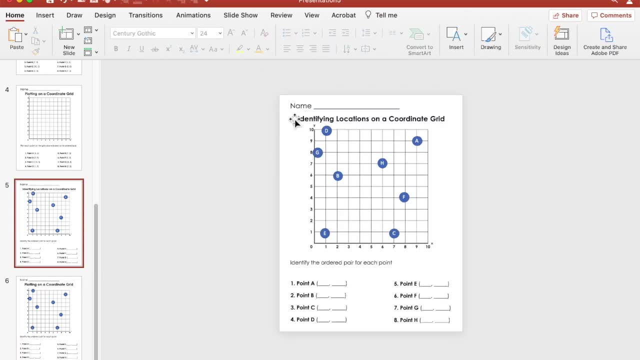 So if you have one to be larger or smaller, that works. We have our saved image. Let me change the title, All right, so I'm going to copy that and bring that over to this one. So now we're going to save it as an image. 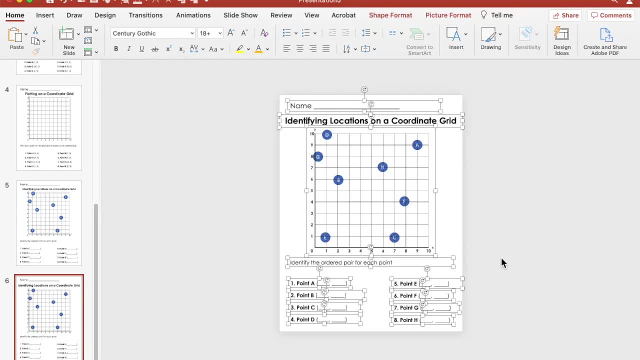 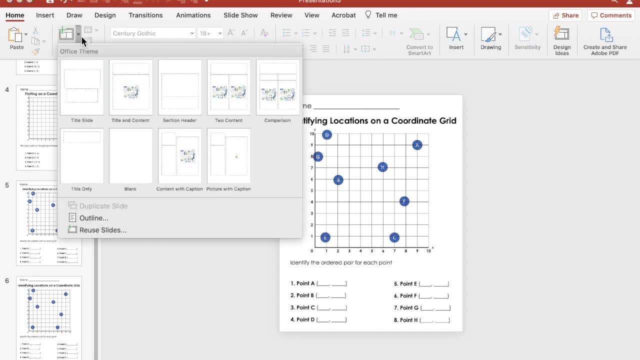 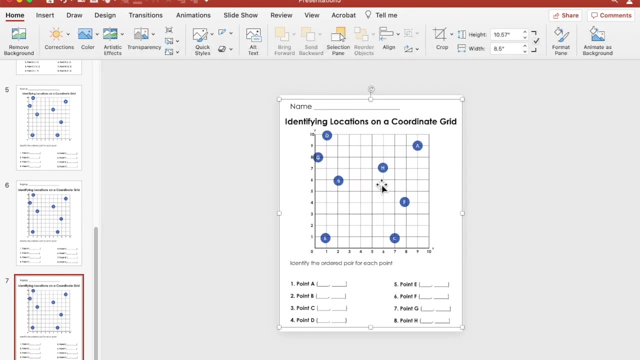 Save, And then we can save it as an image, And then we can save it as an image, And then we can save it as an image. So now we're going to start or do our new blank page and then insert that picture. 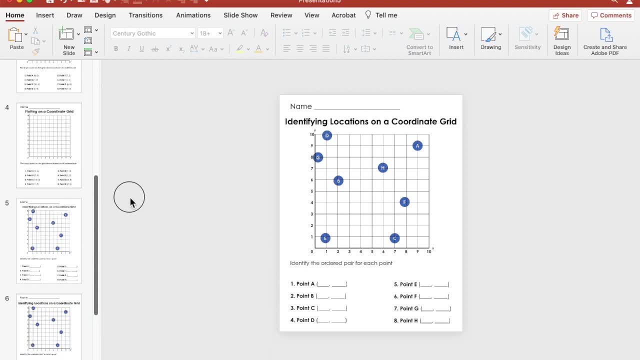 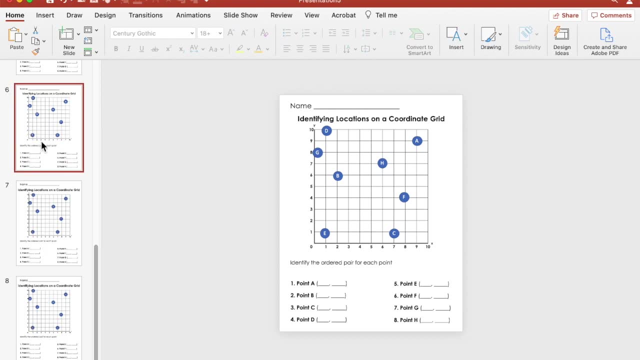 So so far we have two of those pages, So we're going to do one more. I'm going to go back to the original, this one, just because it has that outline. So so far we have two of those pages, So we're going to do one more. 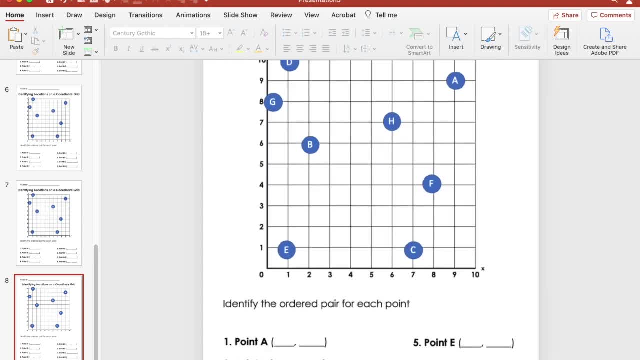 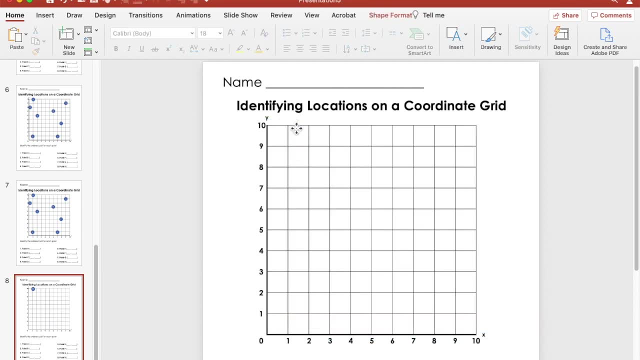 So we're going to go back to the original- this one just because it has that outline- And bring it down here, so I don't mix anything up. zoom in This time, instead of using points or dots, I'm going to use icons that come. 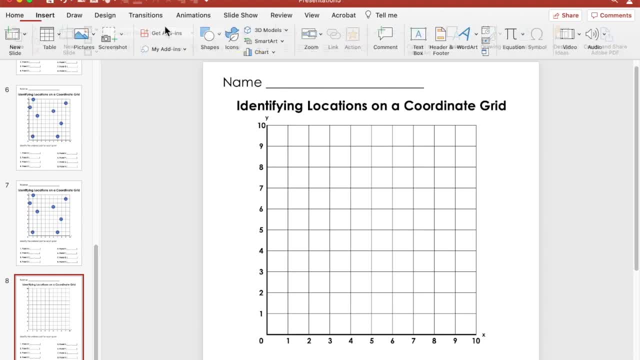 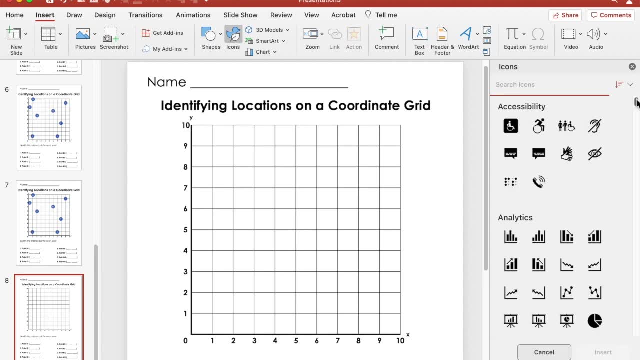 with Microsoft PowerPoint, Go to insert and go to icons. You can also grab images off of the internet, off of Google, off of Bing, wherever you get your images. Let's just use like location So we can do a house and insert that. 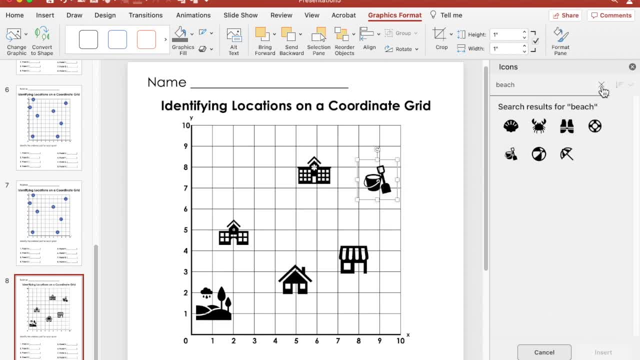 So I think that's enough. There are so many different options you can choose from. You don't have to just do locations. You can do animals, bugs, food items, clothing items. There's so many to choose from. We're going to use these, So I'm actually going to select. 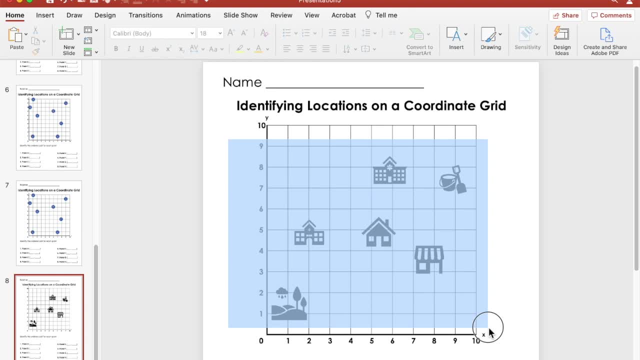 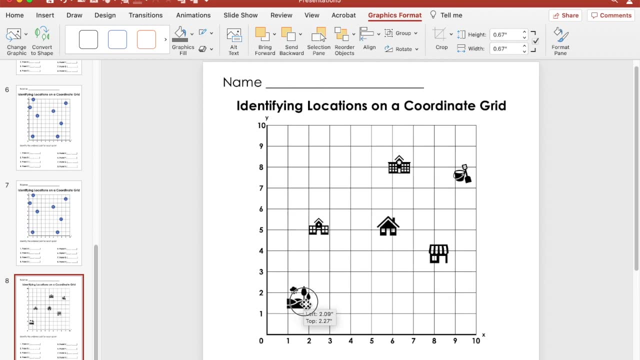 all of them and then minimize their size slightly and then move them around. So I'm going to unselect and then just place them at different spots on the grid. You can leave it in black and white if you want color. Let me show you how to change the color on the icon, So we 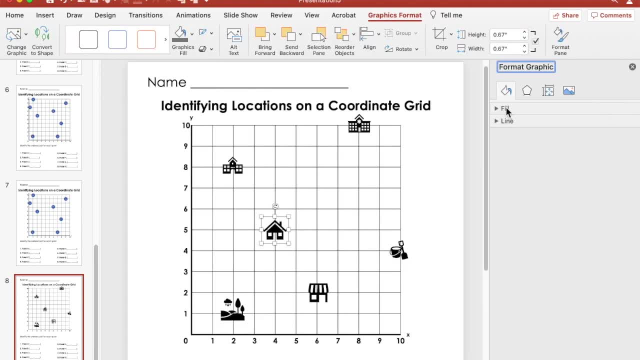 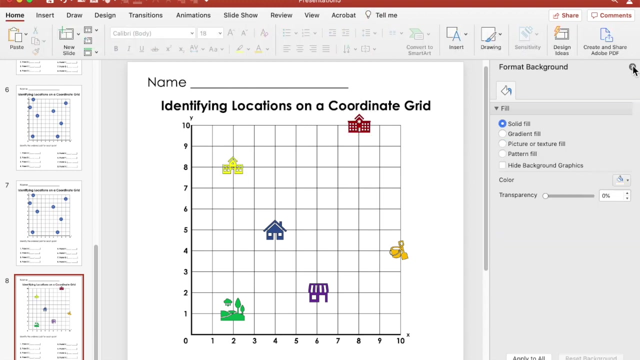 have the house. Just double click that format the graphic and change it to: let's go with the blue, And then I'm going to add an outline For the beach. we can make that orange, Add a line, So there's an easy way to add color to your page, to add images on. there Looks really. 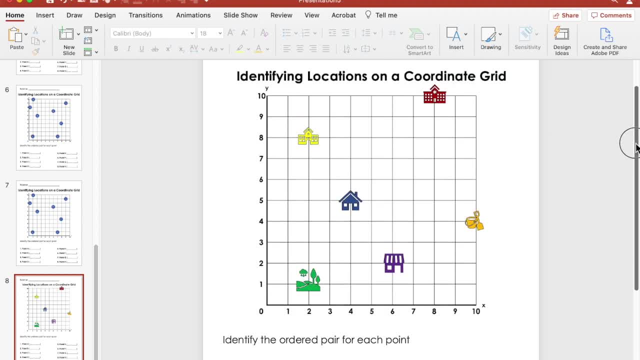 good that way. And you can do it without labels or you can add in labels. So if we wanted to add in a label, you can add another text box or use one of the ones you already have. Just going to bring that in Delete. Let's say: this is the school. 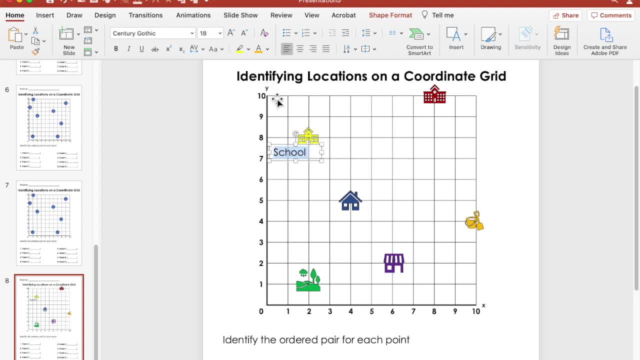 Add another one. Use the one I just made. Add a new one. Add another one. Add a blue one. Add a blue one. Add another one. Add a blue one. Add another one. Add another blue one. Add a blue one. 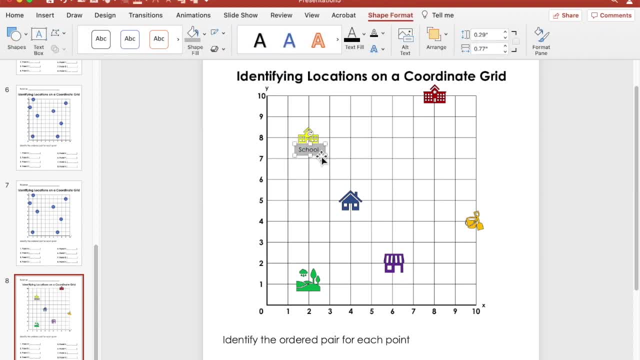 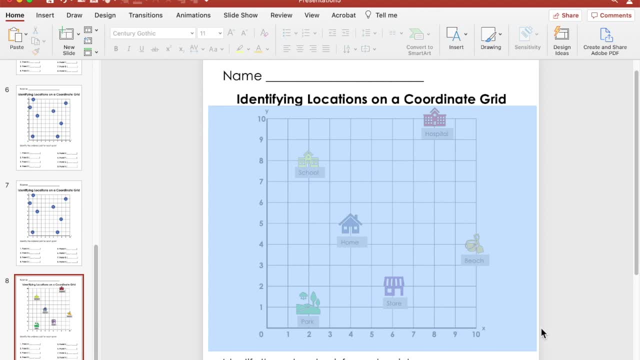 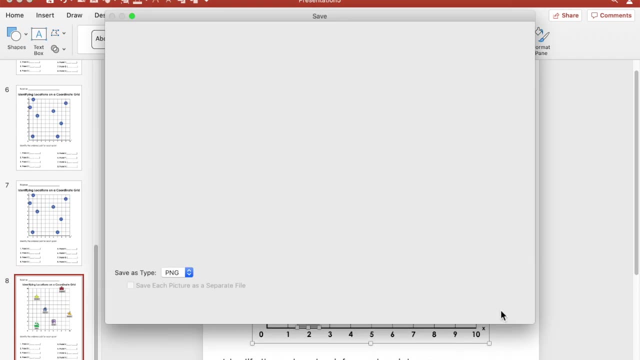 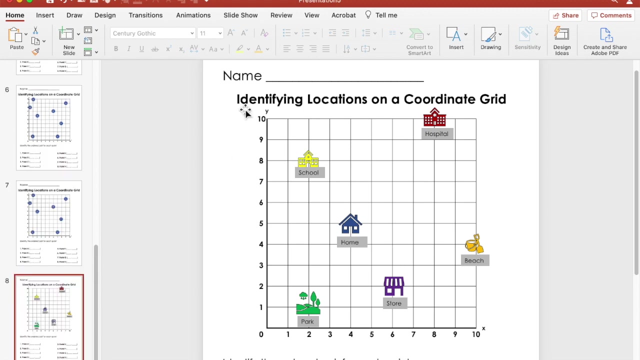 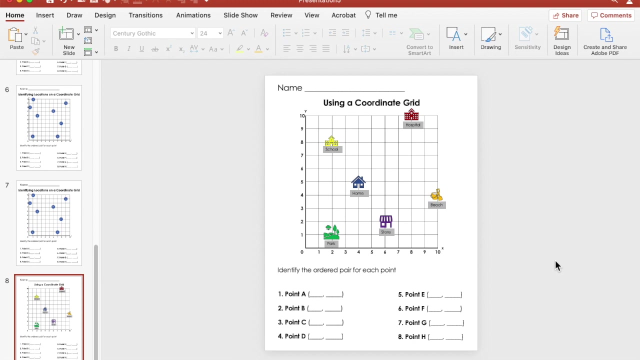 Add a blue one. Add a blue one. now we're going to save this grid with those images, have them all save, save as picture and save. so now, if we duplicate this page, let's go ahead and change, let's change our question so when you have actual images on your page, you can have a little bit more fun with your questions. so 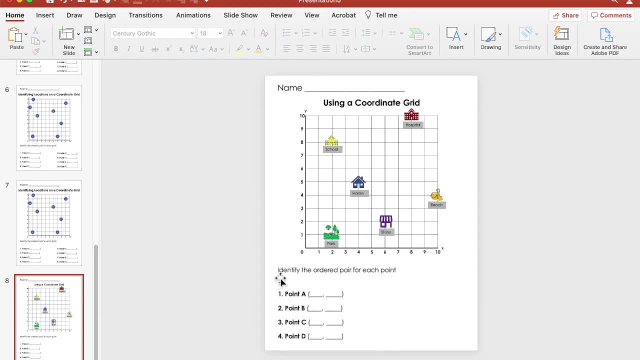 I'm going to get rid of these. I'm going to change the directions and then make these not bold, all right, so let's see. the first question can be: what are the coordinates of the beach question mark? and then you can leave a blank space for the students to write in those coordinates. 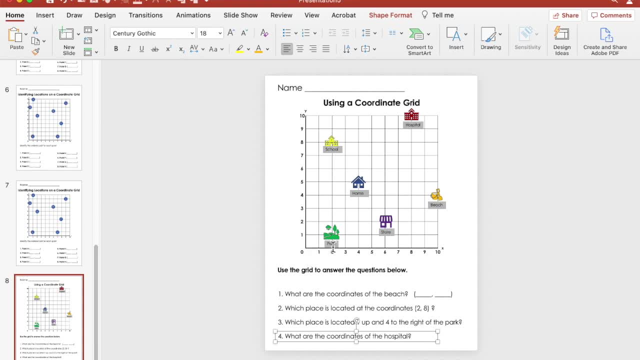 I might make those labels a little smaller, because I don't want students to think the label is where the point is. it's actually where the icon is there. we have our questions to go along with this grid, so I'm going to duplicate it. then I'm going to get rid of the one that we can edit and insert. 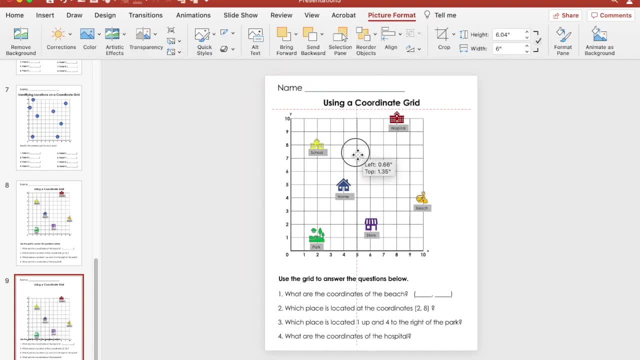 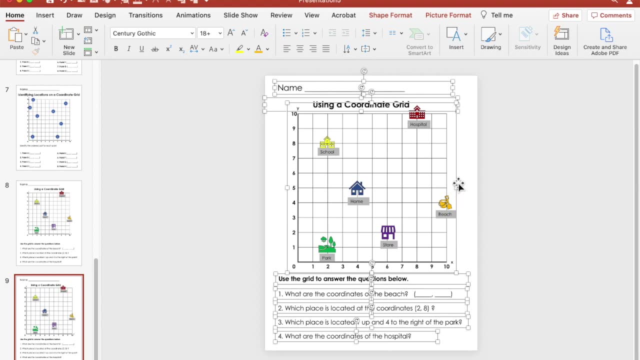 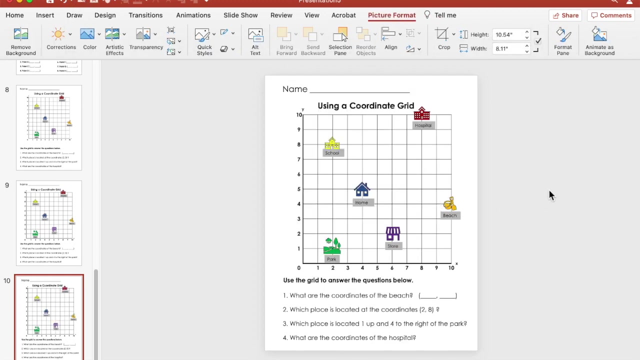 our image that we created and make it a little bigger, and then the last thing I'm going to do is save the entire page as a picture and save that. we're going to put our new blank slide and then insert a page. boom, there you have it. we have our three different pages that we created. 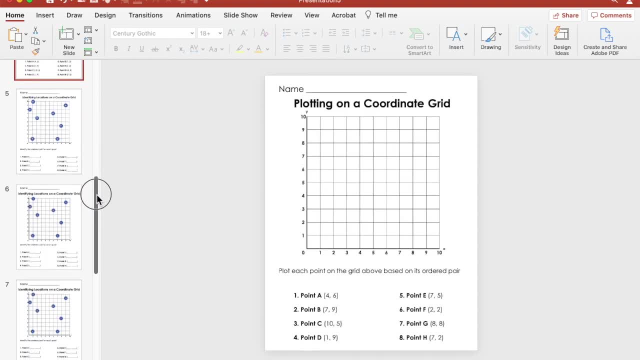 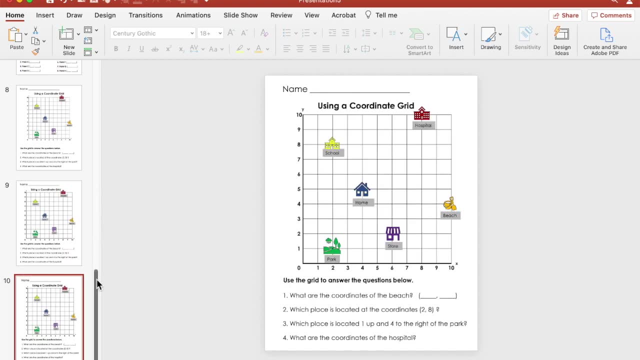 one where the students have to plot on the coordinate grid, one where they have to identify points on a coordinate grid, and then one where they have to answer questions based on the locations of the items on the coordinate grid. so what we're going to do now is save our PowerPoint and save. 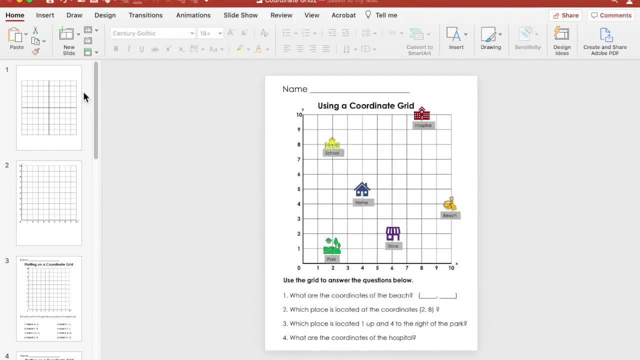 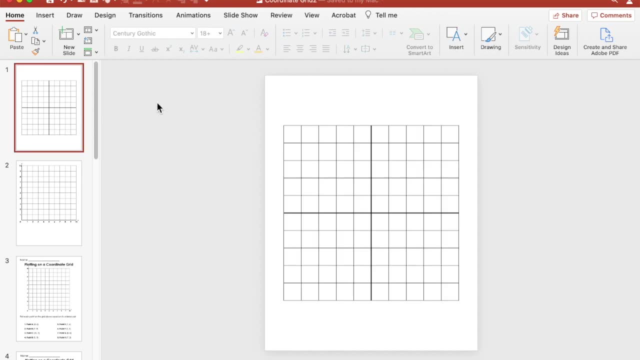 that. so then I'm going to export the pages that I created as a page, PDF, but I don't want my practice pages to go on there. so, because I saved it as a PowerPoint, everything on here right now is already saved, so I'm going to delete them, but make sure I don't 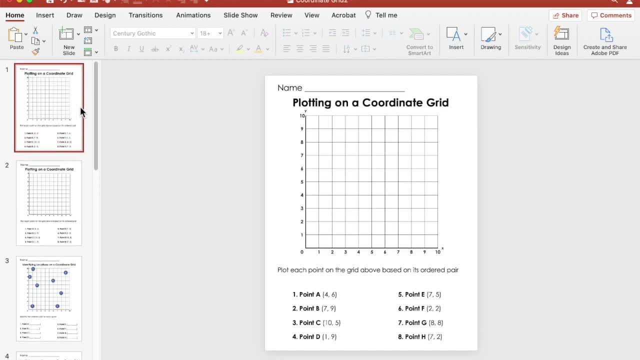 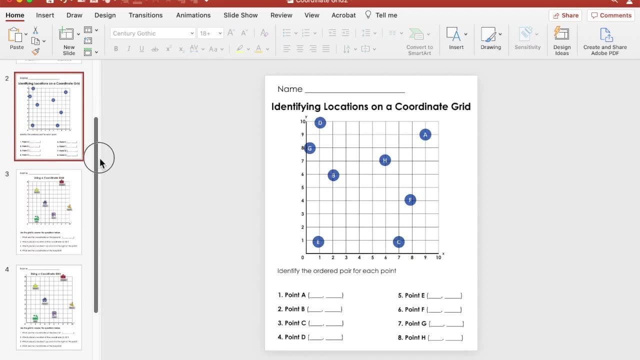 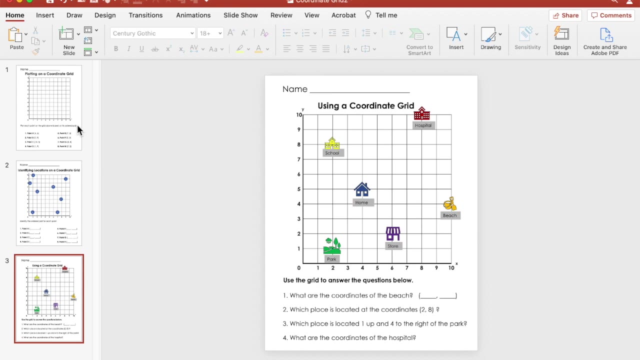 save it again, because I don't want- I don't want them to be deleted on my actual saved page. so I know, the third one for each set is the page that I want. so now I'm left with three, and these are the pick, the, the images that I want, and then I'm going to go ahead and save those pages and then I'm going to